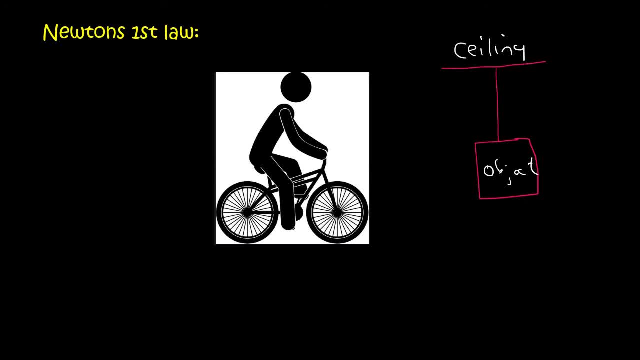 and then here we've got some object. Now let's say it's just hanging there. That means it's not moving. That means that all the forces acting on that object are balanced. Now, what forces are acting on that object? Well, there's gravity that's trying to make it go down. But then there's 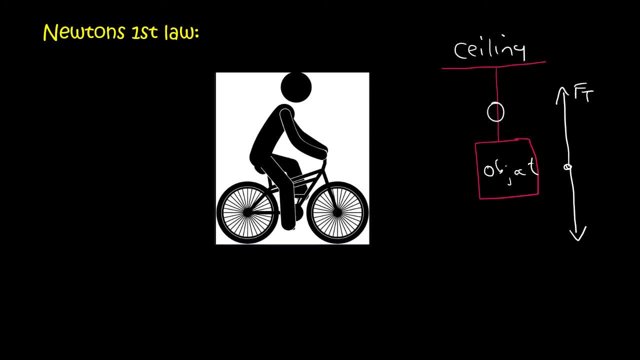 the tension in this rope, And so we'll call that Ft. That's something we haven't looked at yet: Ft for tension and Fg for gravity. If those two forces are balanced, then the object won't move. So we can now summarize. 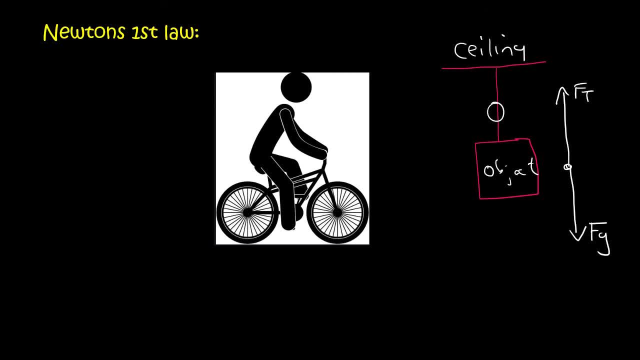 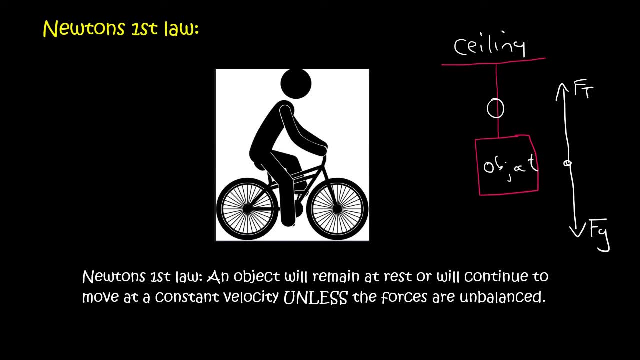 Newton's first law, But remember, I'm summarizing it in my own words- You need to use the definition that your teacher is giving you, And so here it is, guys. Now, remember, my definition is very close to the normal definitions. I just like to phrase it in a way that is easy to understand. So 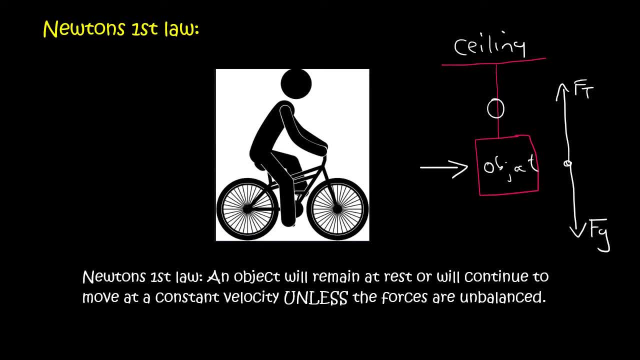 it says that an object will remain at rest. So remember this object is at rest or it will continue to move at a constant velocity, like this guy on his bicycle, unless the forces are unbalanced. So if the pedals or if the force of the person suddenly becomes more than the friction, then the 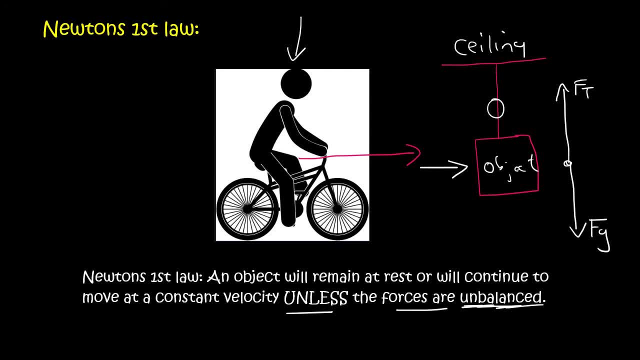 person will start accelerating. They won't move at a constant velocity. If we put a heavier object over here and let's say that this rope cannot stretch any further, then the rope will snap and the object will start accelerating. So let me read it again: An object will remain at rest, such as 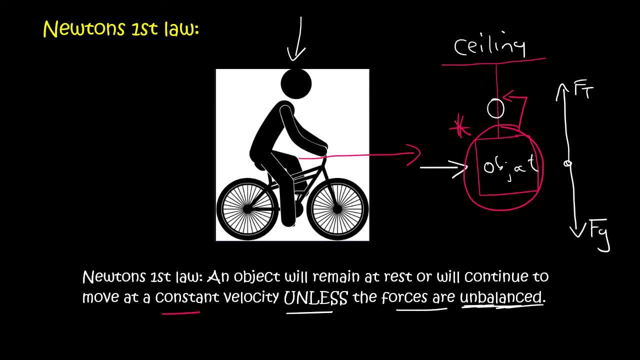 this one, or will continue to move at a constant velocity. Velocity is like speed, And if it's constant, remember 20 kilometers per hour, unless the forces are unbalanced. And so that's all I want to talk about in this lesson- Newton's first law. And so thank you for watching.